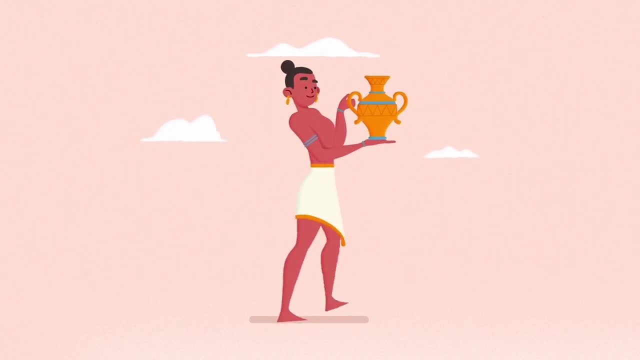 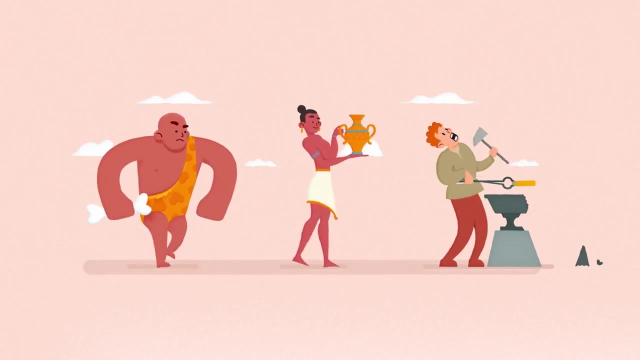 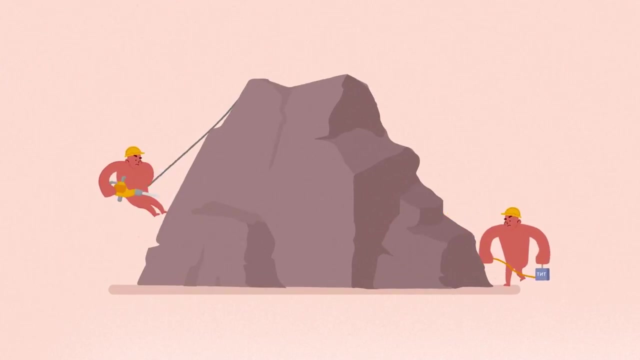 From the Stone Age to the Bronze Age and from the Bronze Age to the Iron Age. The importance of materials has been recognized throughout history. One important attribute of materials is their strength characteristics, and through time, there have been many different tools for measuring the strength of materials. 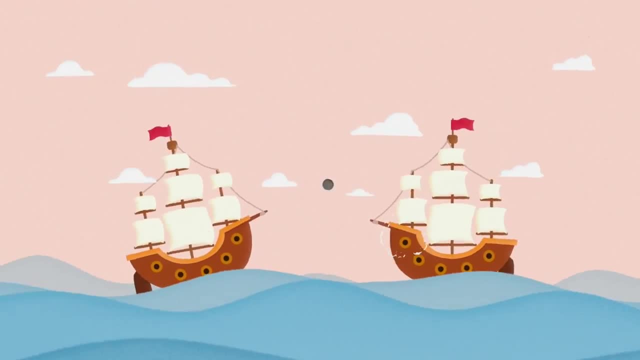 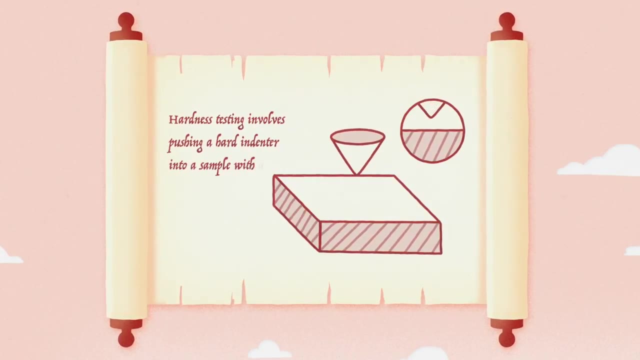 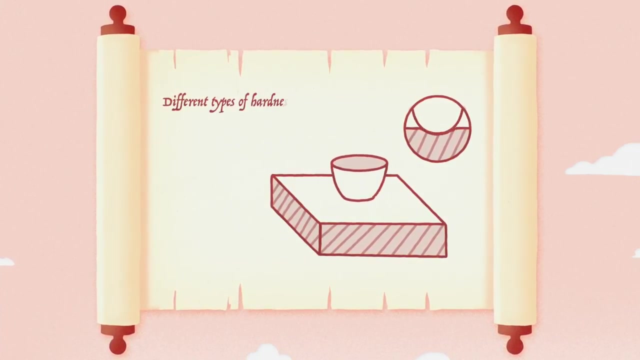 The oldest is the common hardness test, dating back to 1722.. Hardness testing involves pushing a hard indenter into a sample with a known force and measuring the size of the residual indent. Different types of hardness test differ only in the shape and size of the indenter. 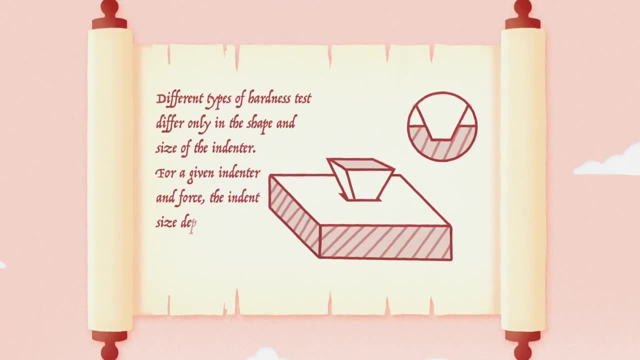 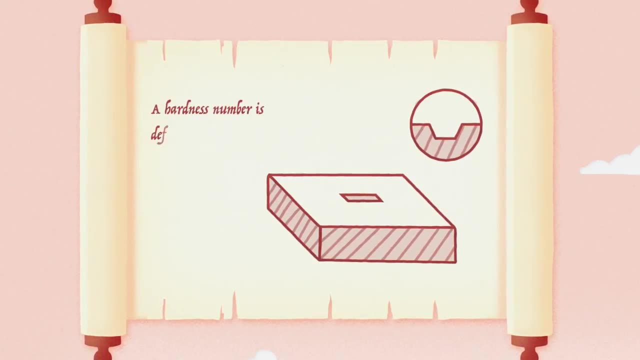 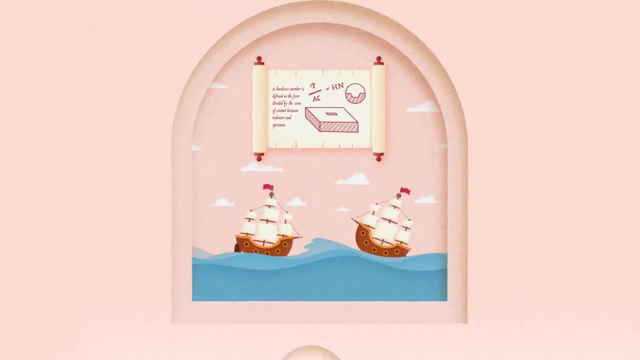 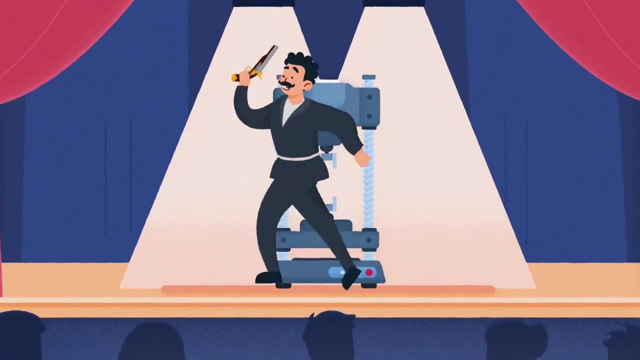 For a given indenter and force. the indent size depends on the resistance of the sample to plastic deformation. A hardness number is defined as the force divided by the area of contact between indenter and specimen. At around 1890, late in the 19th century, early tensile test machines started to become available. 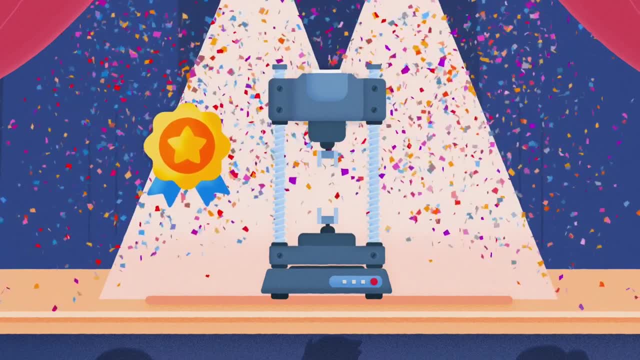 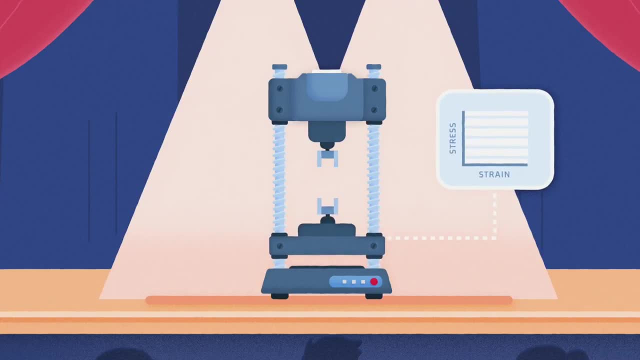 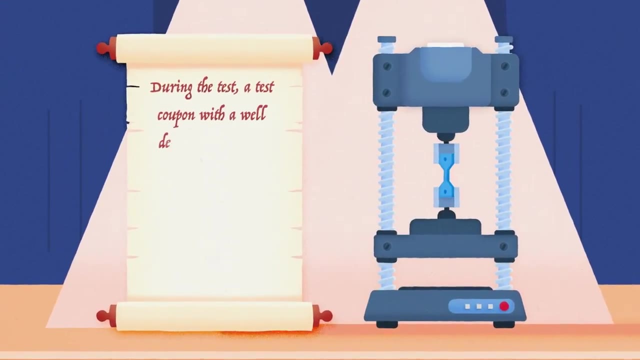 The tensile test has remained, since then, the gold standard in mechanical testing, and it continues to be the go-to method for measuring stress-strain curves. During the test, a test coupon with a well-defined geometry is gripped at both ends before it is stretched under the application of a measured axial force. 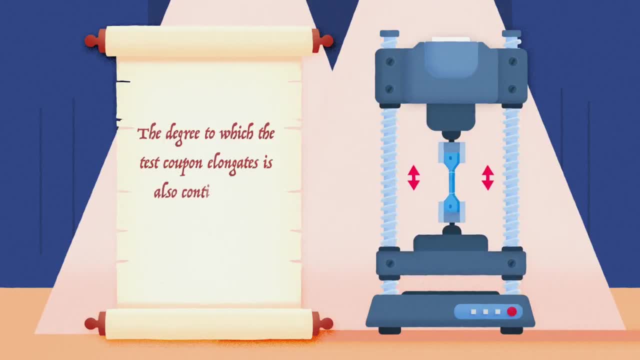 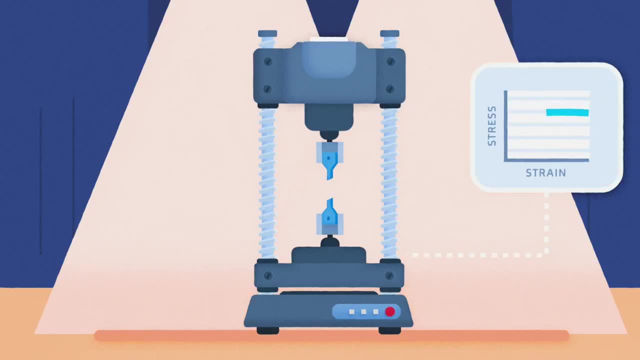 The degree to which the test coupon elongates is also continuously monitored, and when the test finishes, the measured forces and displacements can be converted to stresses and strains, such that the stress-strain curve can be obtained and analyzed. However, tensile testing also suffers from some limitations. 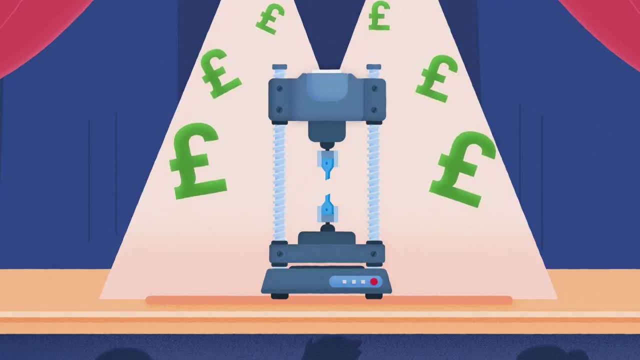 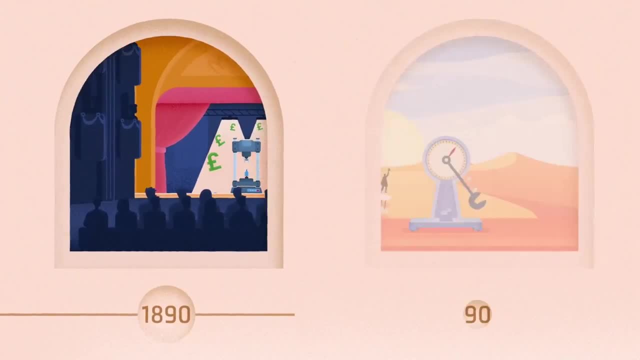 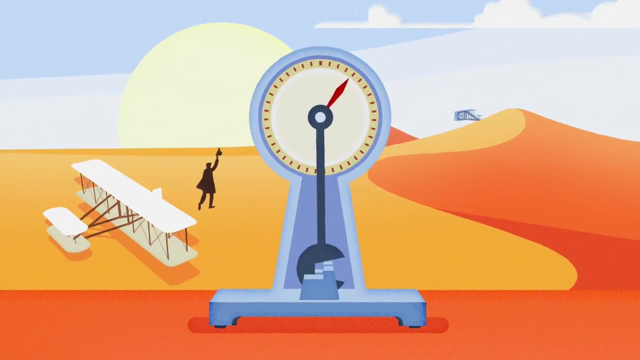 including capital investment costs, coupon preparation difficulties and clamping and slippage challenges. Also emerging at about the same time- 1901, was the Charpy impact test for measuring the fracture energy of materials. The test technique is popular because of its simplicity.